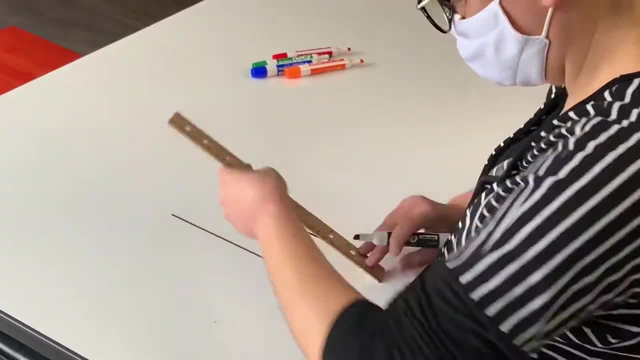 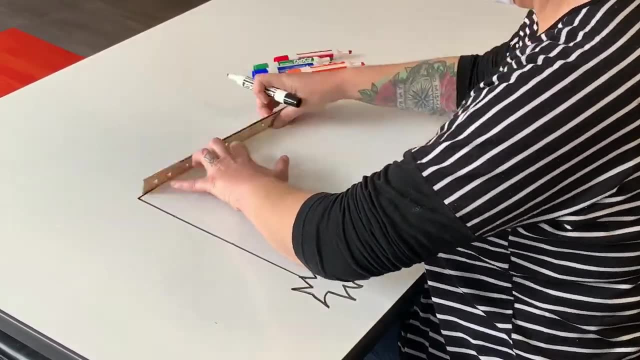 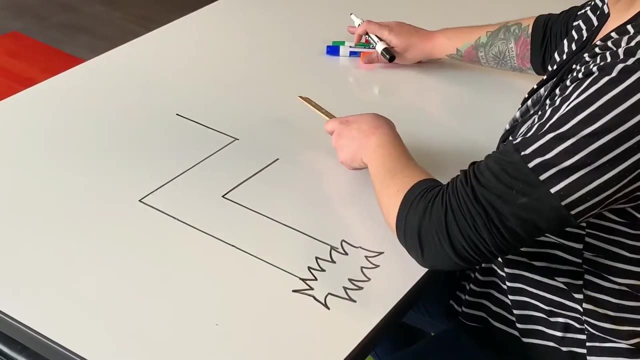 so the first thing you are going to design is your board. The idea is that you create a board with as many spaces as you like and in each space you are going to write a math problem. Remember to write the board with a start and a finish line. that's very important. 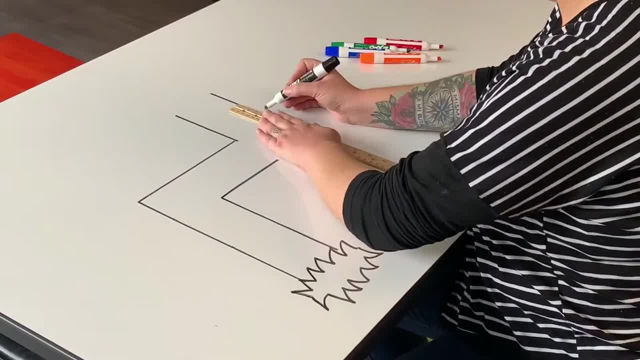 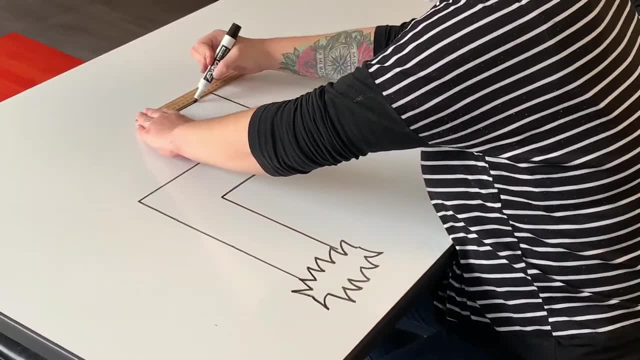 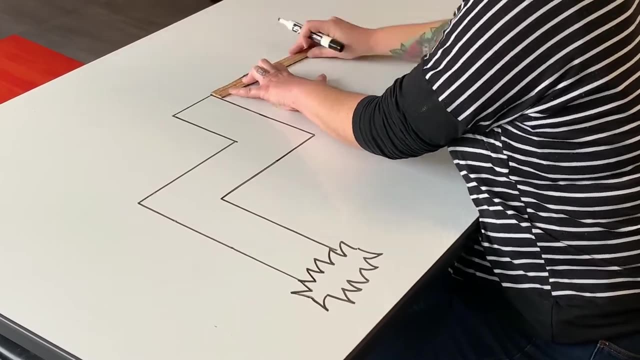 And as far as the equations, you can do some subtraction, multiplication, division. the choice is up to you And of course it will depend on the math level where you feel comfortable at To write the equations. you should ask for the help of an adult. All right, so I'm doing some of the spaces here. 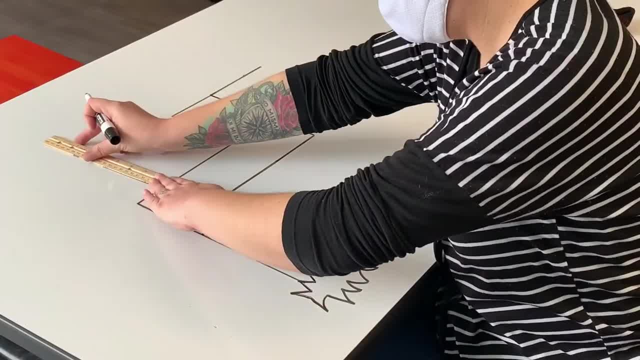 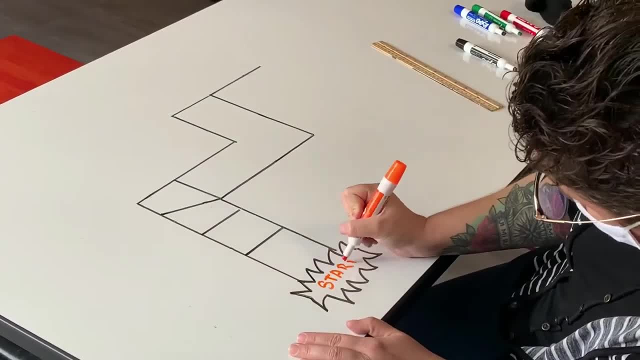 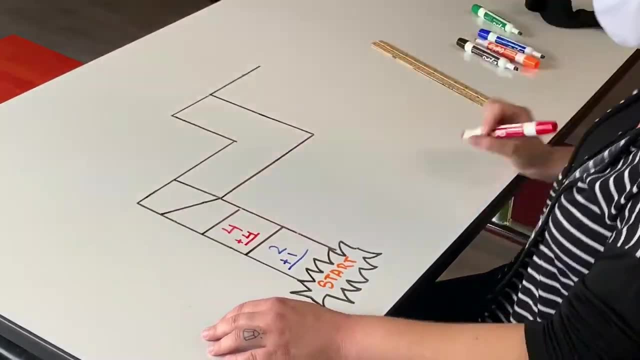 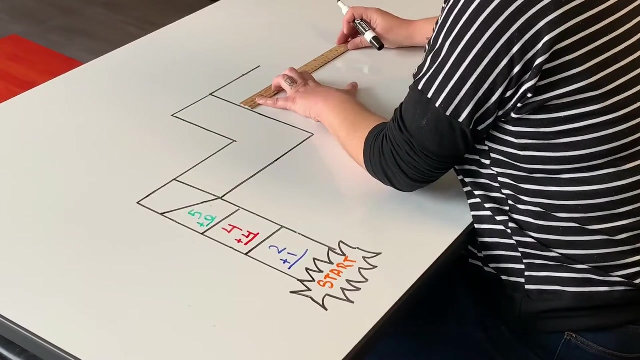 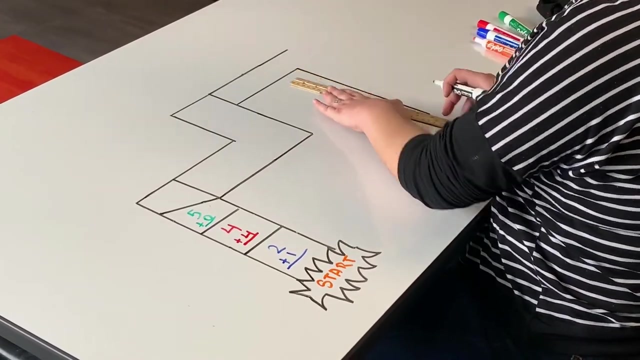 As I told you, you can do as many spaces as you like. I have my start line and I'm going to start the equations Today. we're just going to do some 해�おい. Remember you can't write the solution because you can't write the solution to the. 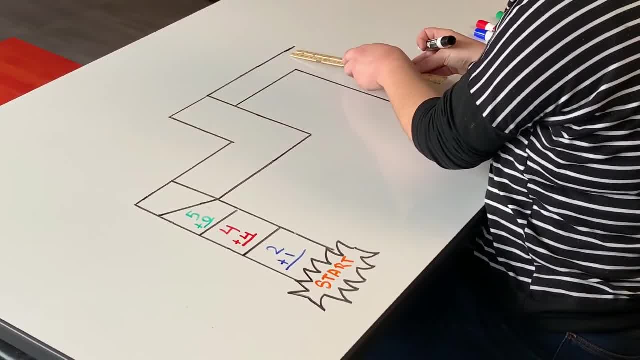 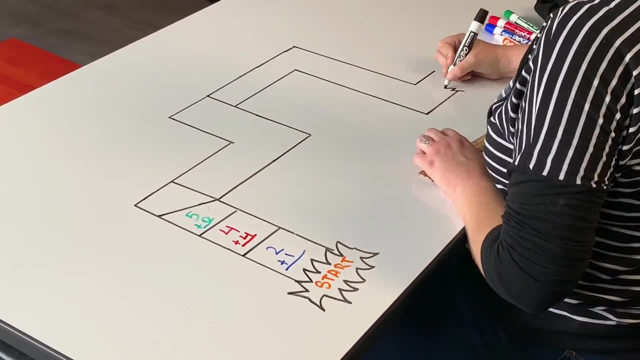 equation, because the whole point is that whenever you're at one of the spaces, you're going to solve the problem, And you can do this in paper or cardboard. We did it on this big whiteboard just so it's big enough for everyone's home. 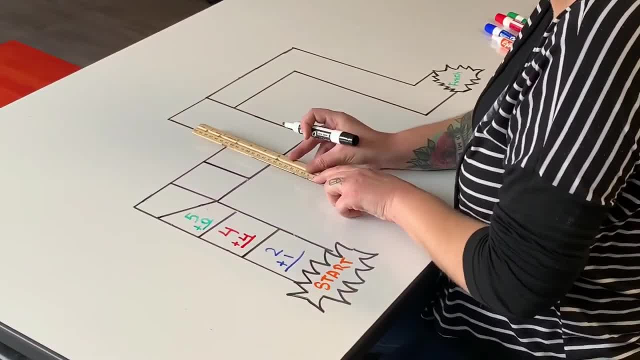 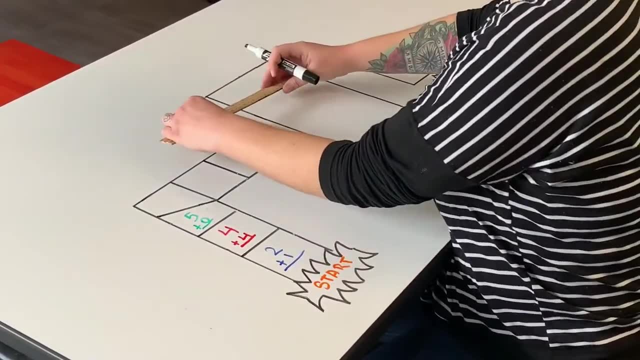 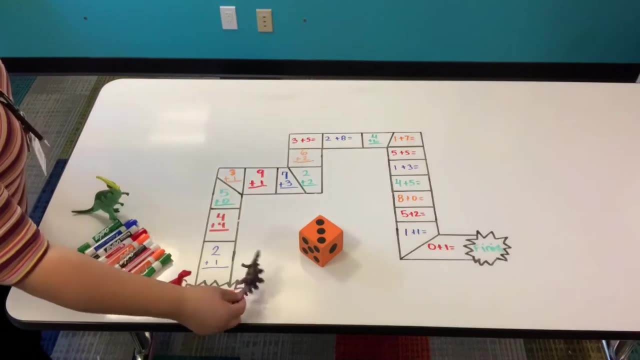 just so it's big enough for everyone to see through the camera. Also, we use different colors, so that way it looks a little bit more fun. Okay, so it's time to play, and we got our pawns here. Natalie and I are gonna play. 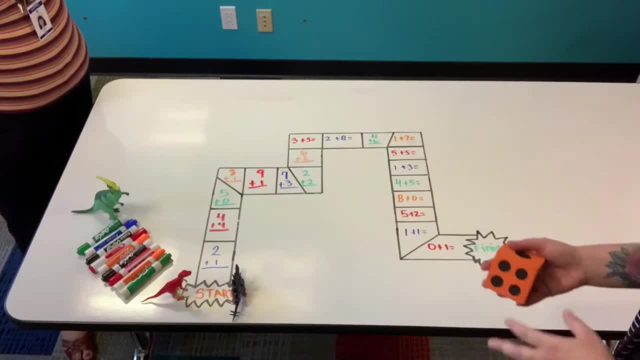 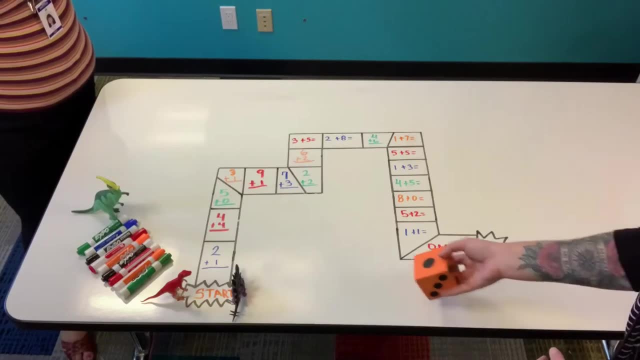 and the first thing we're gonna do is we're gonna roll the die each of us, and whoever gets the higher number it's gonna get started. All right, let's see I got three. Let's see what Natalie gets.